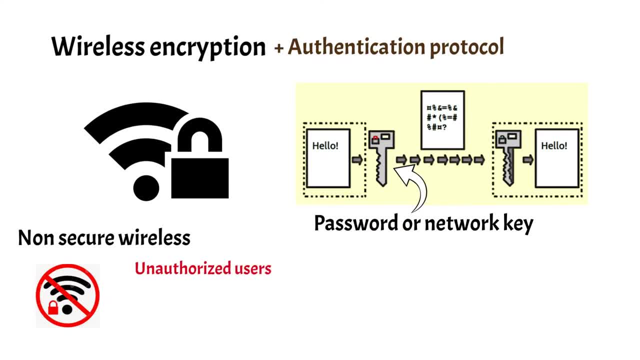 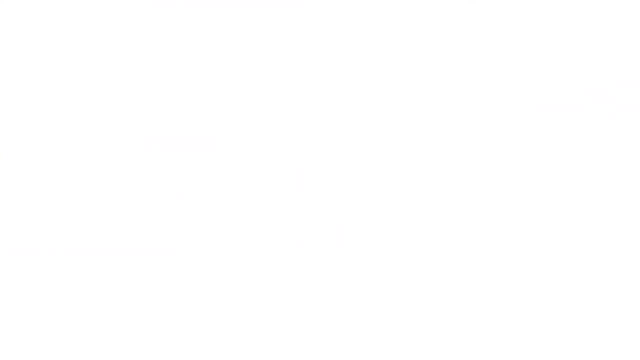 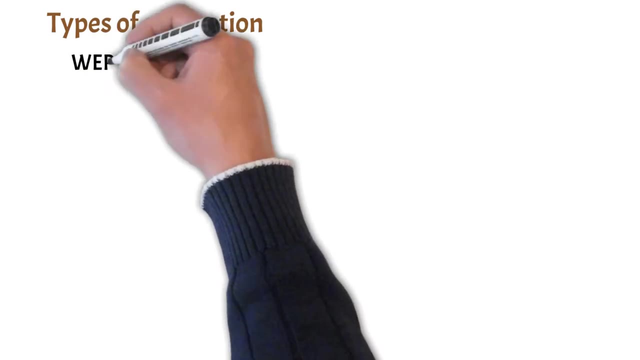 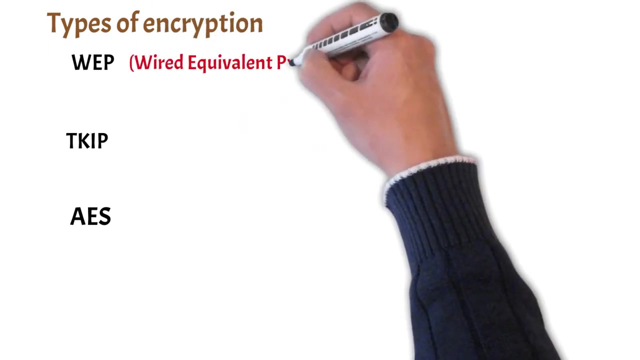 access your network and obtain personal information or use your internet connection for malicious or illegal activity which can degrade your network performance and speed. Following are the types of encryption available for wireless network: It has WLANs, WEP, TKIP and AES. WEP, also known as wired equivalent privacy, uses the RC4 cipher algorithm. 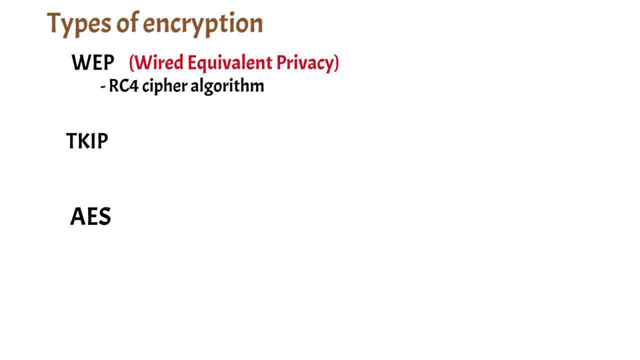 to make every wireless data frame private and hidden from eavesdroppers. The same algorithm encrypts data at the sender and decrypts it at the receiver. WEP is considered to be the weakest of the available encryption methods. Then we have Temporal Key Integrity protocol. It was originally created in order to help. 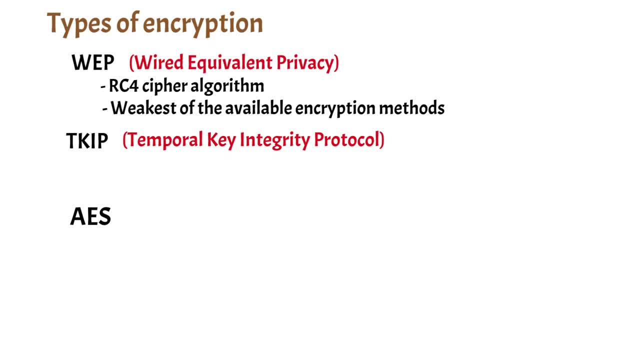 address the natural shortcomings found with the WEP encryption. It uses the same RC4 encryption algorithm. However, TKIP is more secure and has an additional feature called Message Integrity Check. MIK is designed to protect both your network and your internet connection. Just like the. 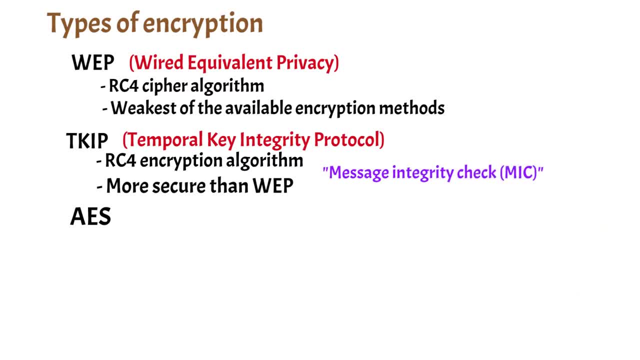 same Jewish network. it receives the same sort of encryption for your network and is used in both of your devices, not just for your devices. denk duns ID and IP contracts also keys, data payload and header. prevents network attackers from conducting bit flip attacks on encrypted 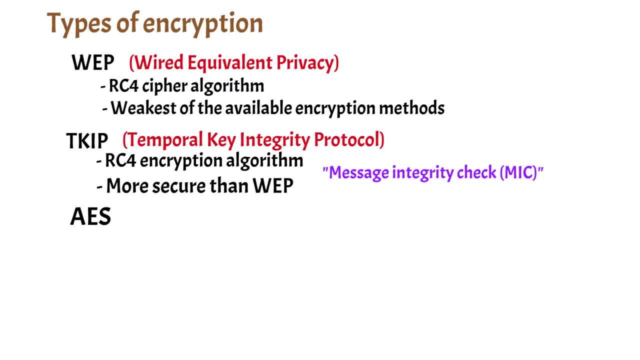 network traffic. during this type of network attack, an intruder will first intercept an encrypted message, then he or she will alter the message and retransmit the data packet. mick help prevents this type of attacks. then we have aes, also known as advanced encryption, standard encryption algorithm. 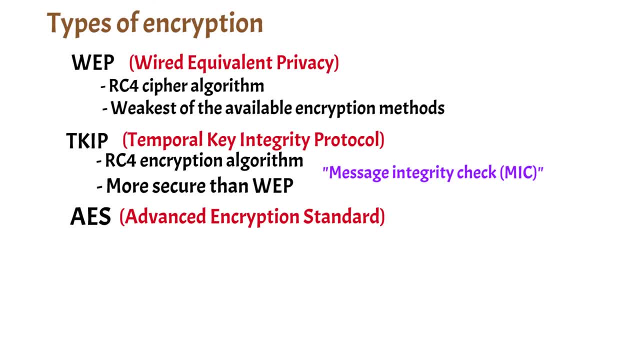 a widely supported encryption type for all wireless network that contain any confidential data. it uses reindahl algorithm and is considered significantly stronger than rc4. aes provides a high level of security and is the encryption of choice for the us federal government and nasa. it is considered to be the most secure and fast method available for network encryption.